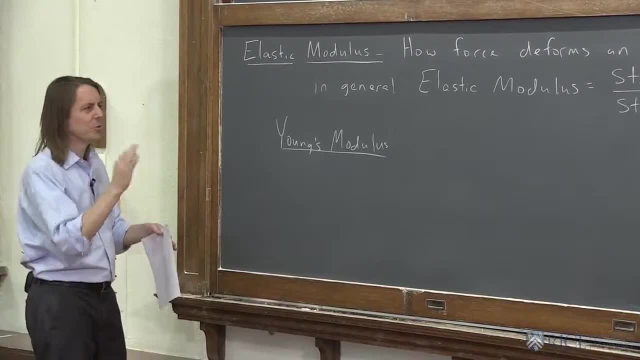 Often they'll just throw words around. They'll say, oh, elastic, modulus, And sometimes they'll call it Young. Sometimes they won't. So I was trying to tell you there's the general way to think of it, And now here's the specifics. 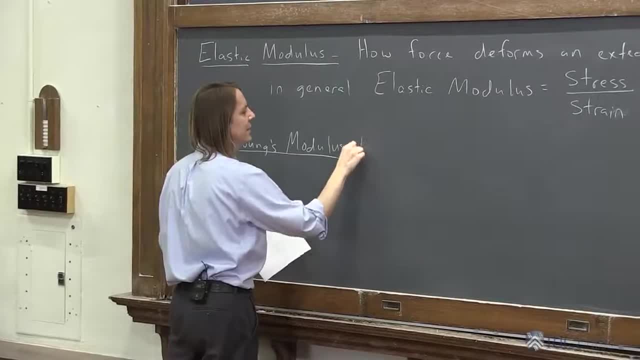 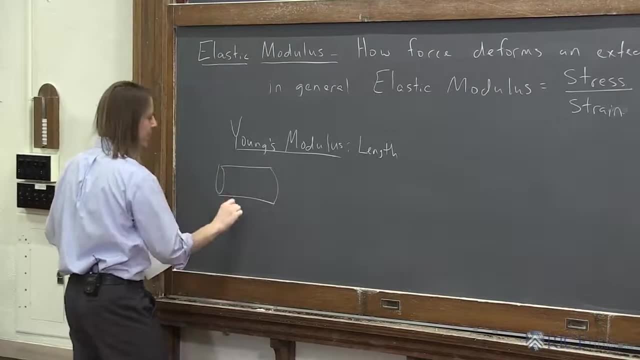 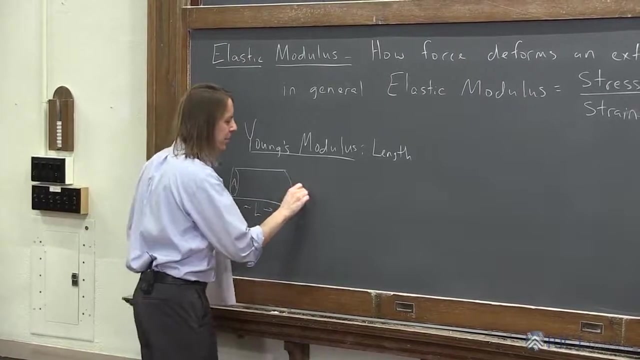 So Young's modulus is usually when you're extending the length. So say, I have a rod of some material that looks like this And it's got a length L And it's got a cross-sectional area A If I apply a force to it. 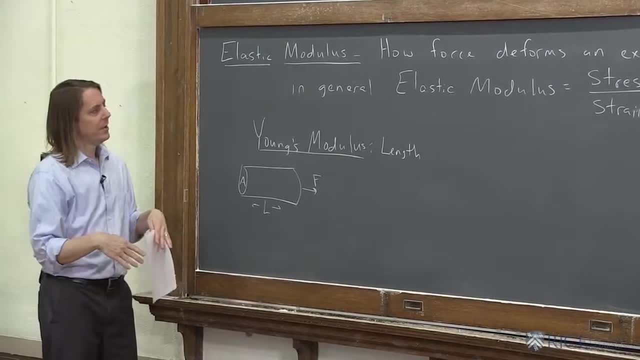 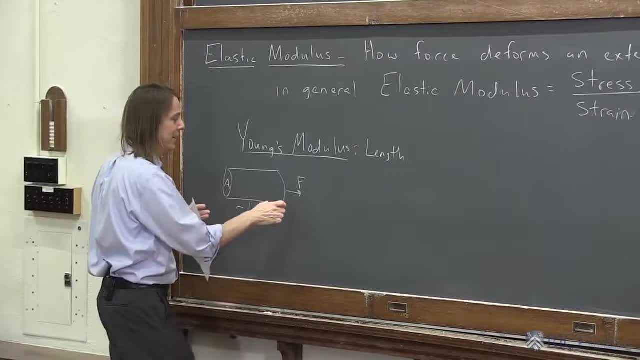 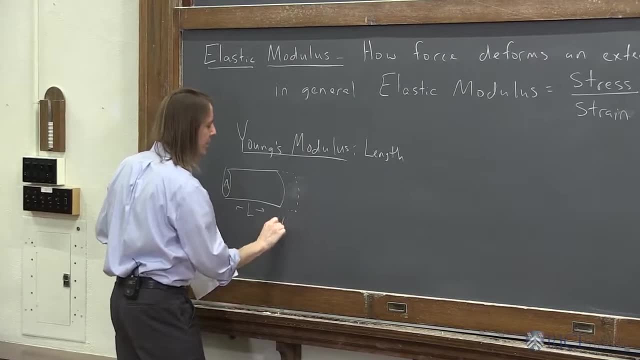 Nothing's going to happen, But in reality a real material. if you pull on it it'll stretch, So it's really. then we pull and it gets a little longer, like that. We'll call that delta L, So we pulled on it. 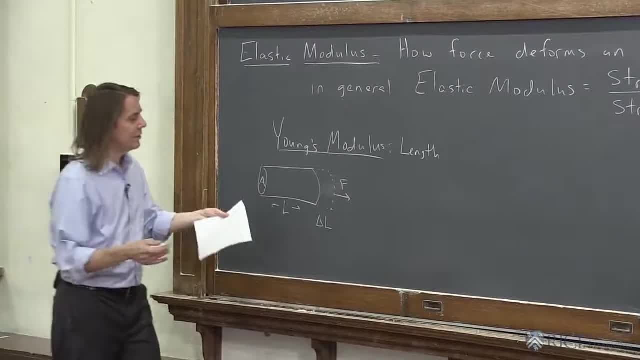 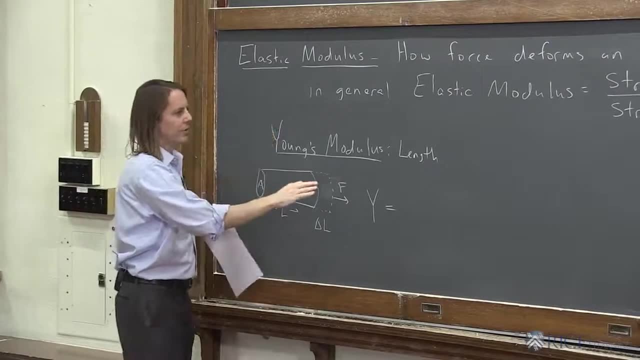 We made it longer. So this is just the equation that describes that. There's this thing called the Young's modulus y, And it is the stress over the strain. The stress is the force per unit, So it's got the unit of a pressure. 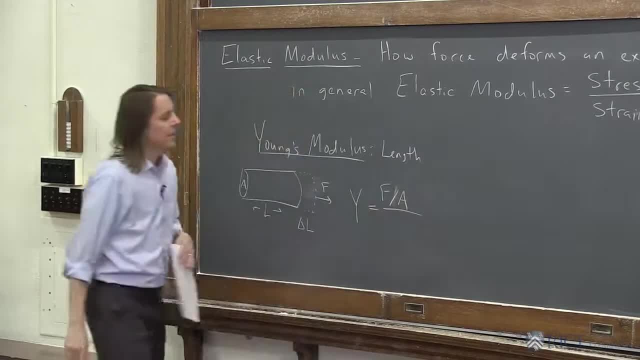 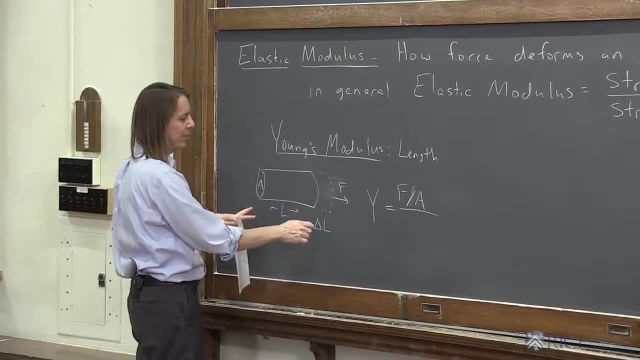 It's kind of like a pressure force per unit area, And the strain is a unitless description of how deformed it is. So the clear way to make it unitless here is: take your delta L and divide it by L. It's like the fractional extension. 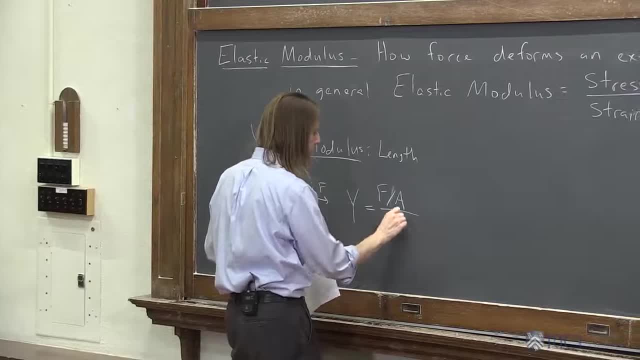 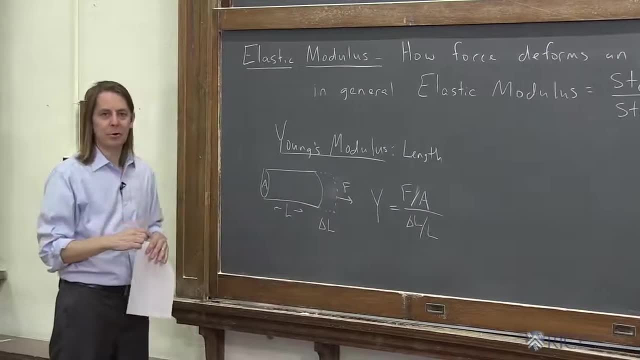 or the percent it extended or whatever you want to call it. So delta L over L, like that. So in the end the unit of the modulus is a pressure. It's Newton per meter squared, but it's really more than it's. 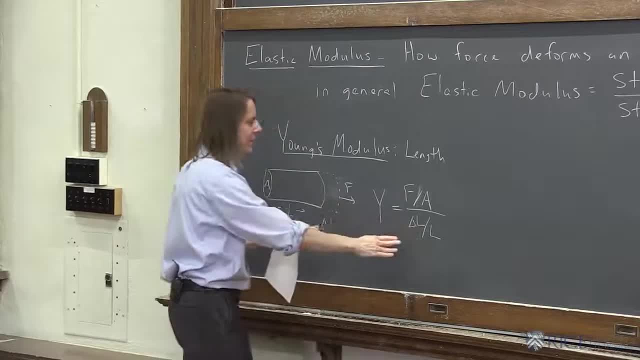 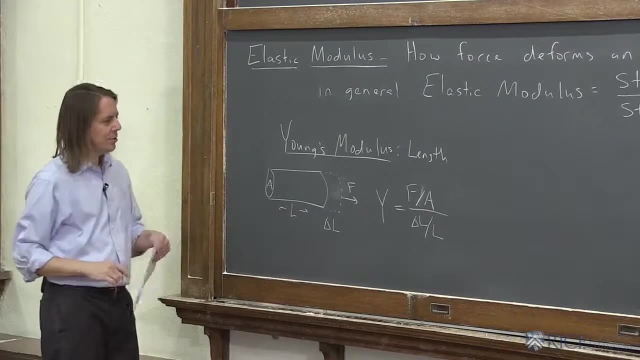 not really a pressure. It's a description of how that pressure extends the object in a sort of fractional sense, which is why meters don't show up in that sense. So we'll use some of these and you'll see sort of how this. 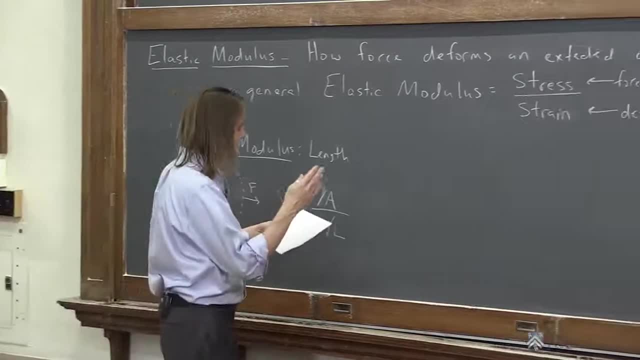 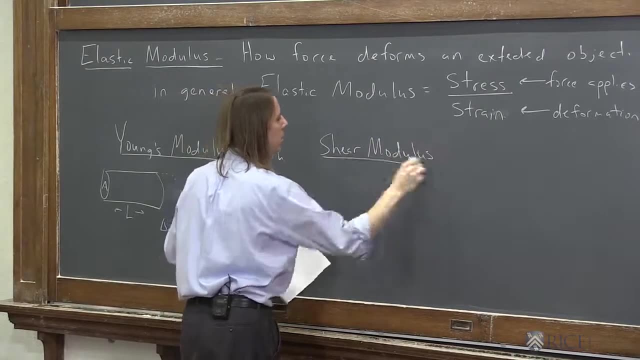 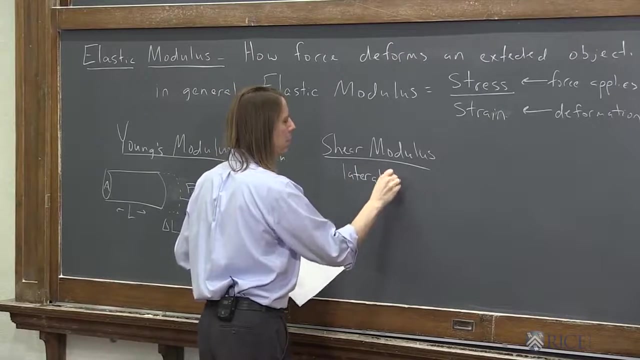 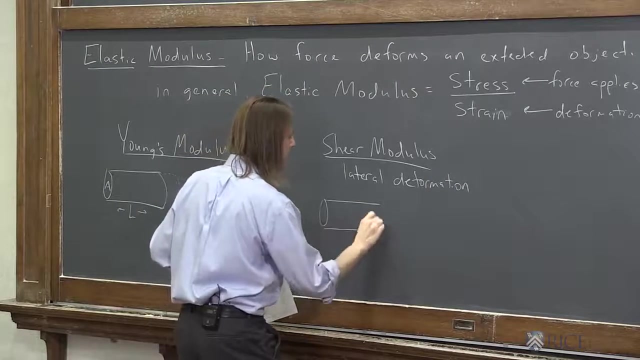 works. But that's for length. But you can also look at shear, so the shear modulus like this, And this would be for lateral deformations. So let's say you have that same rod like that same area, A same length, L like that. 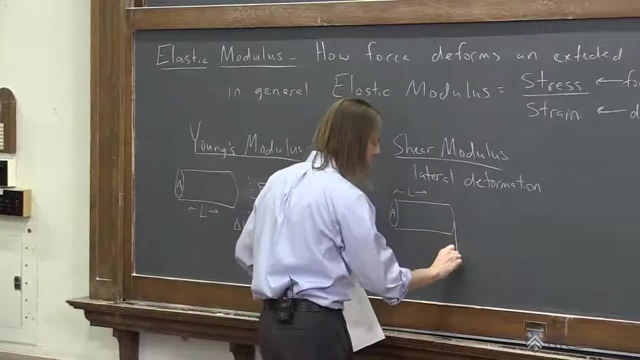 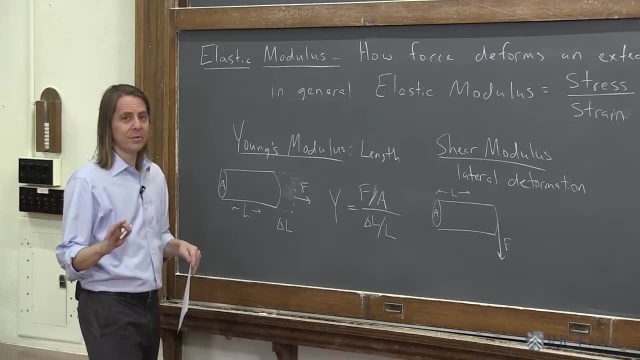 What if you apply the force this way? So you apply the force like this to the edge. What's it going to do? Well, actually, it's going to do sort of two things, And we only care about one of them. So for now, since we're defining shear modulus, 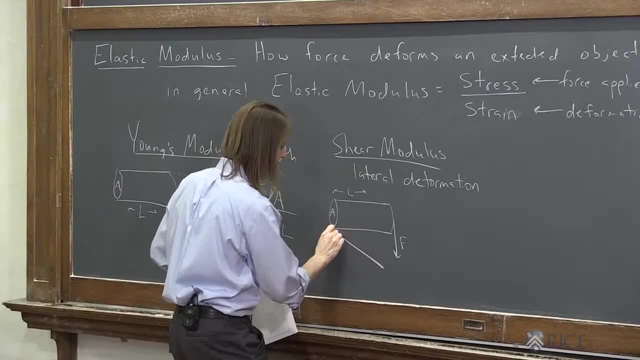 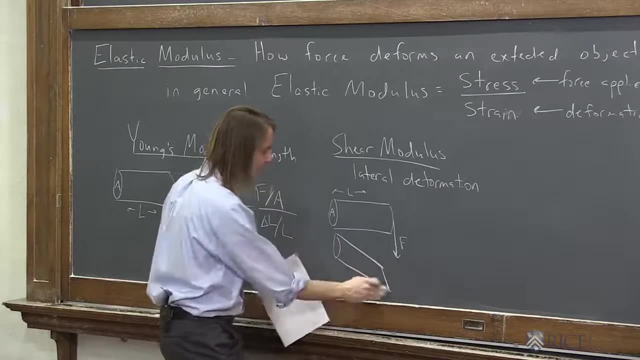 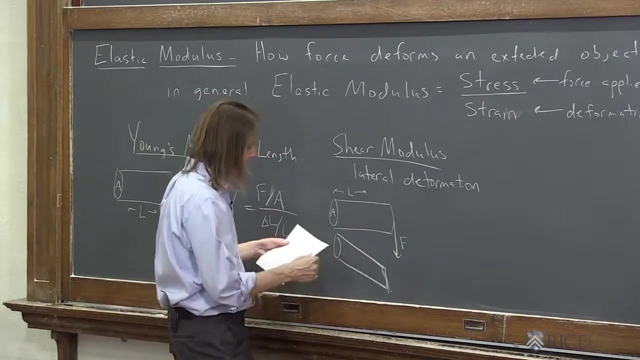 let's say it'll do this, It'll become sheared. OK, All right, So this area will be the same, but it will deform in a way, kind of like that, Like all the slices of the thing will just go down in a shear deformation. 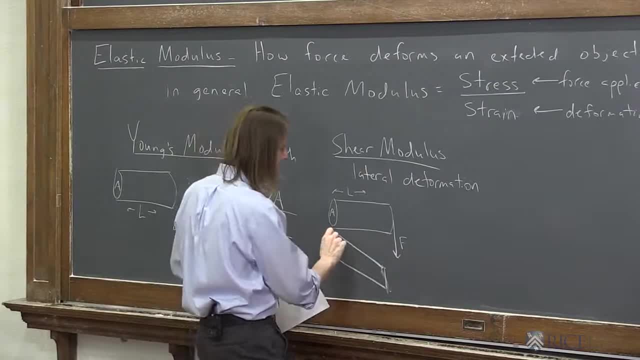 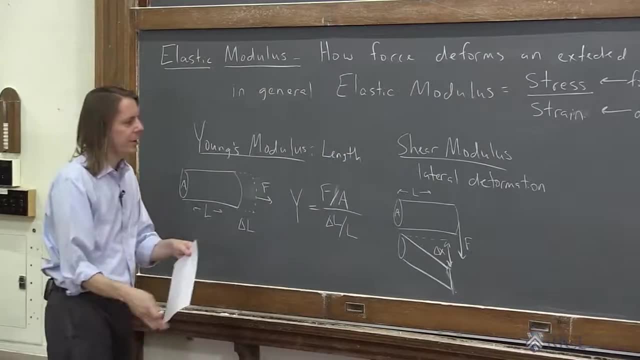 And then the delta L we care about is from where the height of that top edge was delta x. How far down did you shear it? That modulus, we'll call it, I think, S usually, And it's the same. 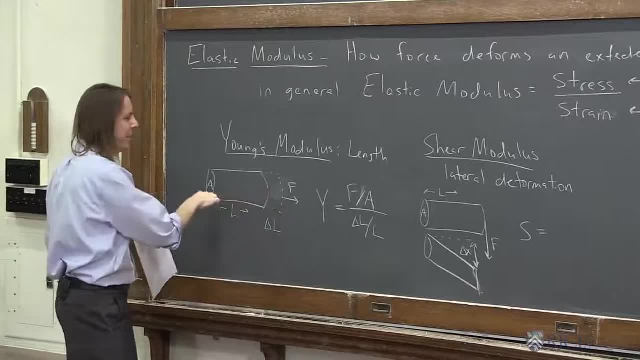 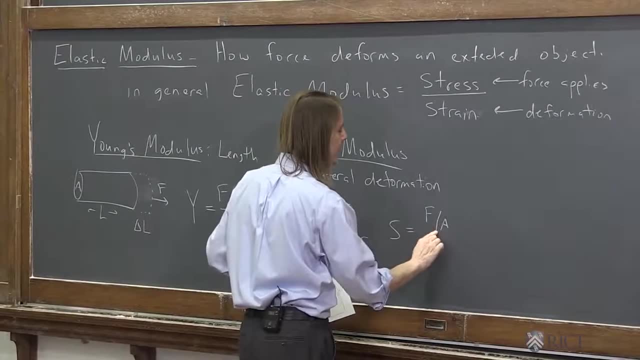 It's the same pressure that you would apply Same force per unit area. it's just in a different direction. So now you can see it's not really a pressure right. Force per unit area, So the same force over the cross-sectional area. 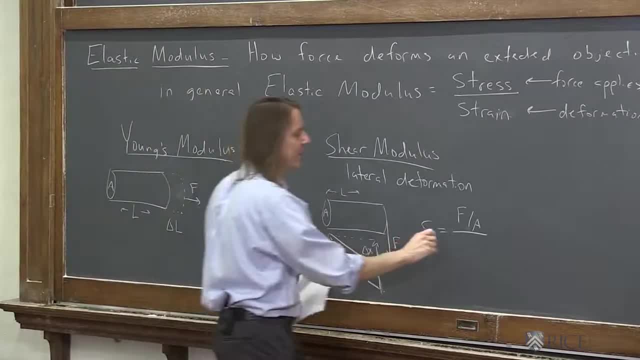 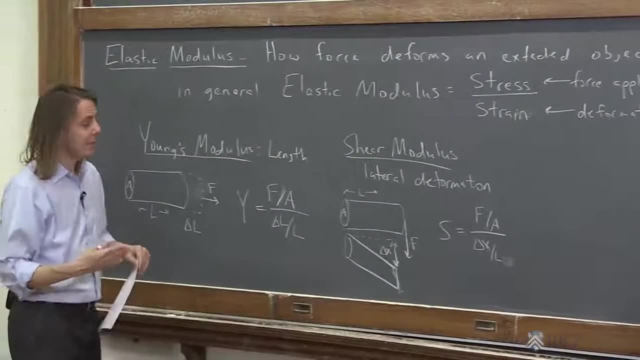 And then again it's a fractional deformation. It's delta x over L, Also a unit of pressure. but you can see it is not a pressure, It is a modulus. It describes how much something deforms. What's a little weird about this one? 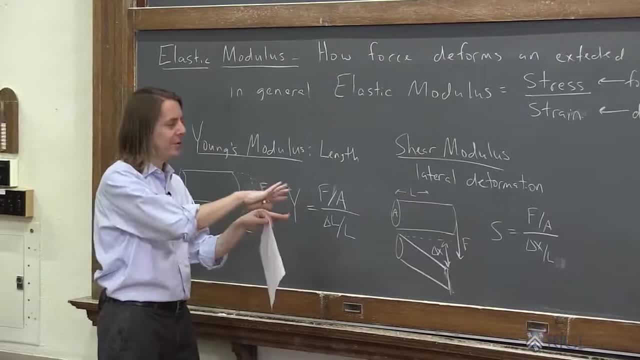 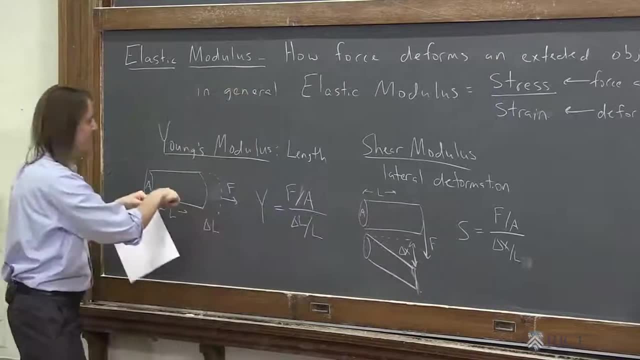 is, if you apply a force that way, it'll also bend, It'll also make a little bit of an arc, It'll partly shear, It'll partly bend, And the bend where it makes like a curved arc is actually this happening If something extends more on the top? 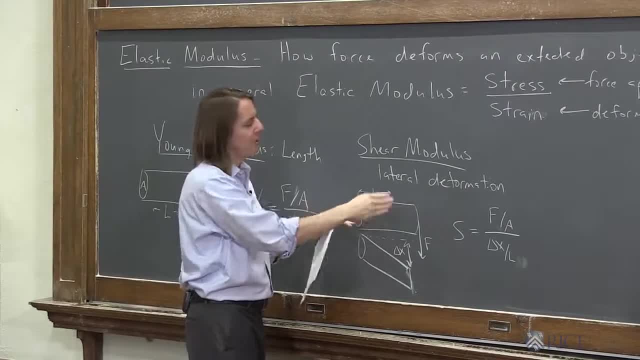 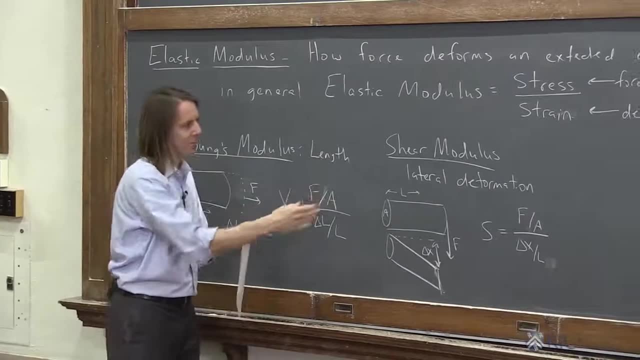 and it contracts on the bottom. it makes an arc. So how much it does that and how much it shears depends on the relative values of y and s. Most materials tend to make an arc, But there is a concept of a shear that can happen. 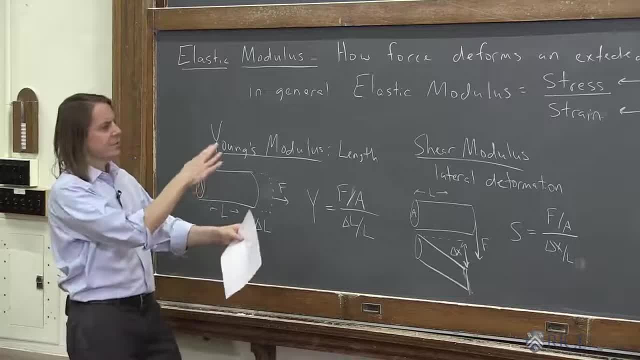 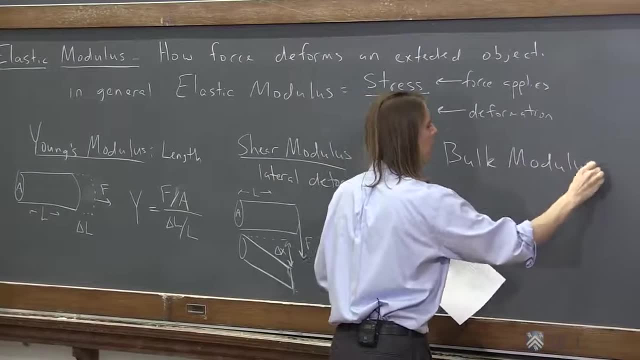 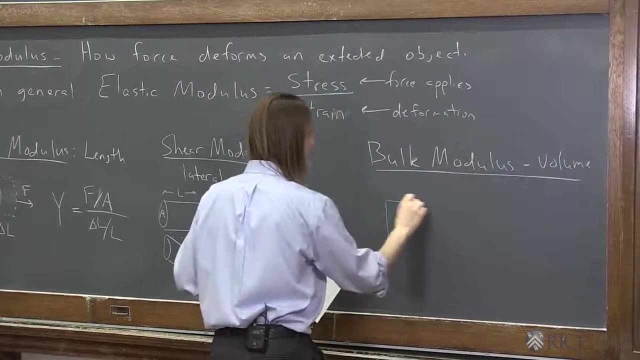 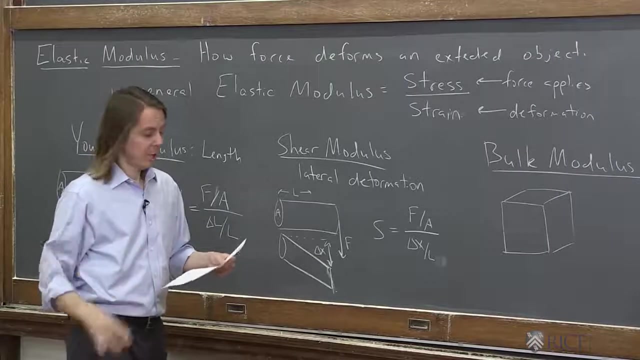 and can be measured. The third one I want to show you, just to get this general picture going, is the bulk modulus And it is for volume. So let's say you have a nice cube of material here And you apply a huge pressure to it.